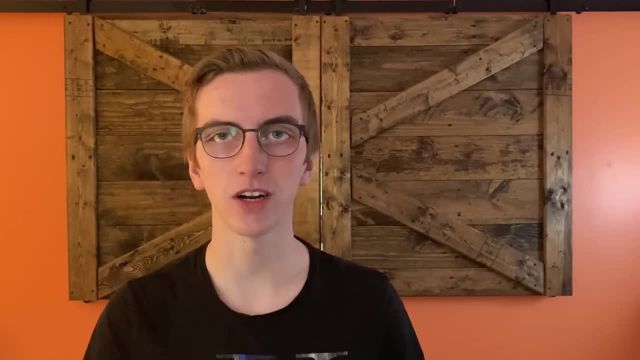 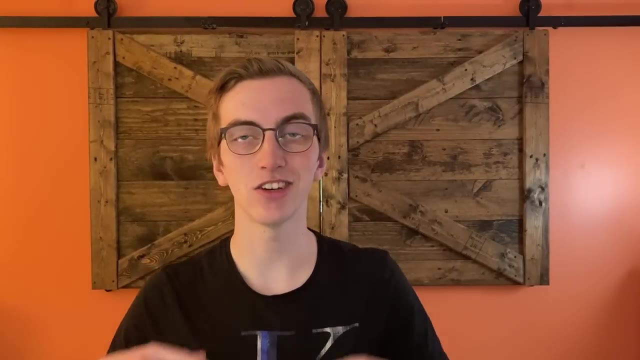 Being underemployed means that you're working a job that does not require a bachelor's degree at all. However, this isn't just an engineering problem. If you look across the United States and Canada, there are tons of people that are underemployed. 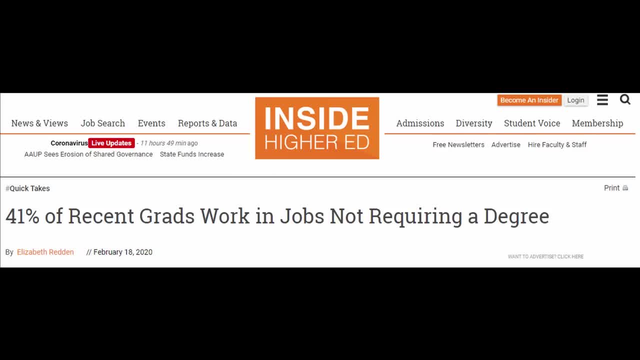 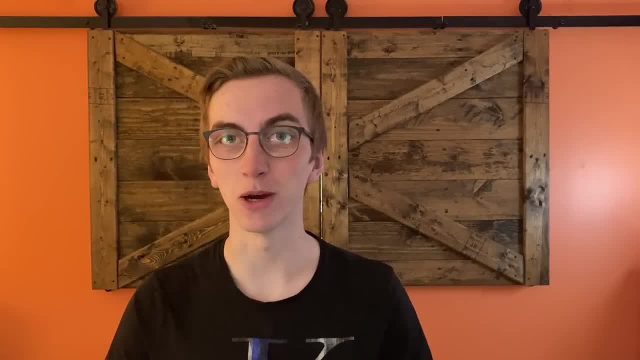 with a recent statistic pegging it at about 40% of people with bachelor's degrees. Okay, so that's a pretty crazy number. I'm gonna come back to it in a minute, but first let me tell you about my sponsor. Ha, just kidding, I don't have a sponsor. 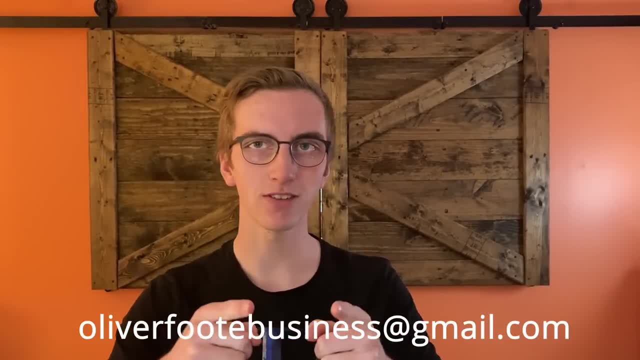 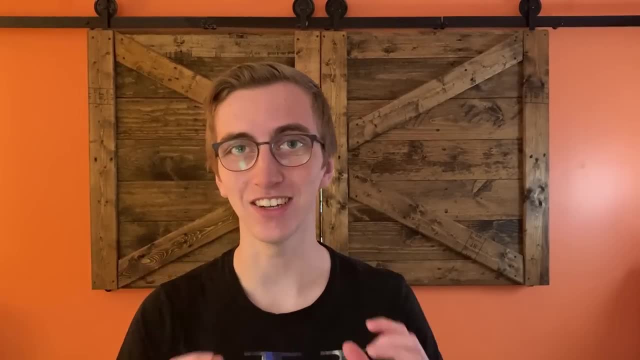 But if you're interested and you want to sponsor me, shoot me an email Now. the fact that 20-30% of engineers are underemployed is pretty bad, but that's not the end of the problem. As I said at the beginning, 75% of engineers are not employed in engineering. 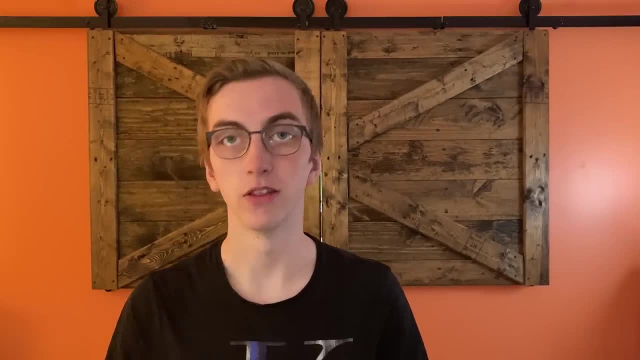 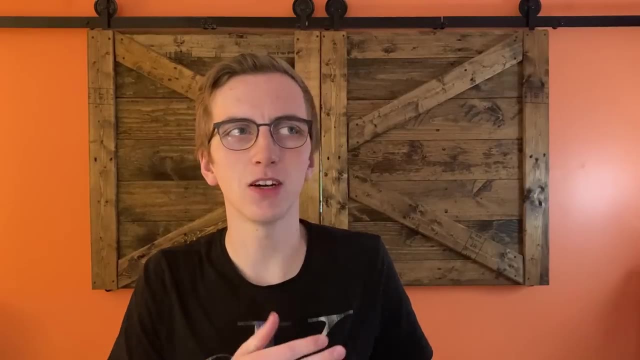 leaving 25% who are actually employed in engineering. This means that 50% of engineers who are employed are working decent jobs, but not engineering. Now, for them, this might not be such a bad thing, because maybe they wanted to work in a different field or they found a job. 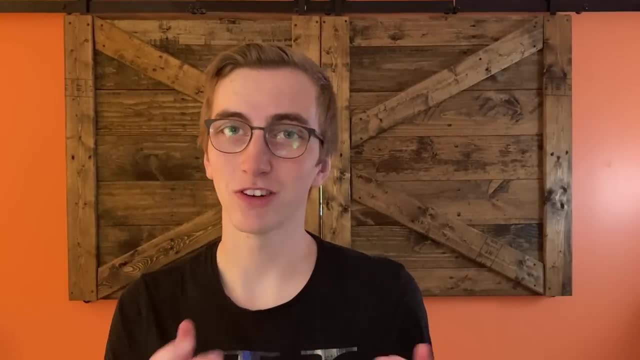 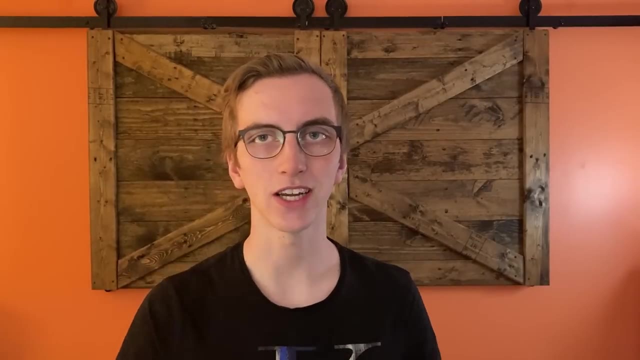 that really interests them. This raises a problem because people with degrees other than engineering are starting to get displaced by engineers. This is a multi-layered problem and I'm not gonna tell you to not get an engineering degree, but I am gonna tell you to think about something other than university. 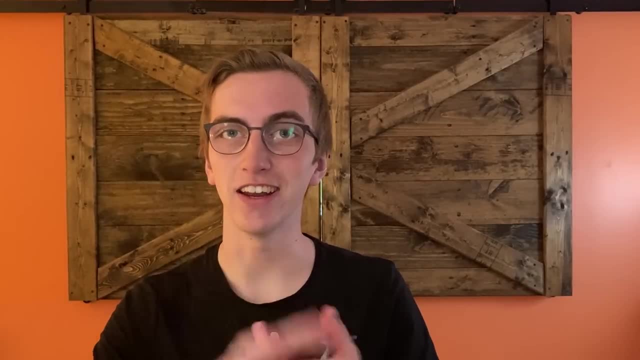 This is a multi-layered problem, and I'm not gonna tell you to not get an engineering degree, but I am gonna tell you to think about something other than university. That being said, if you're dead set on university, engineering and any other STEM field are still. 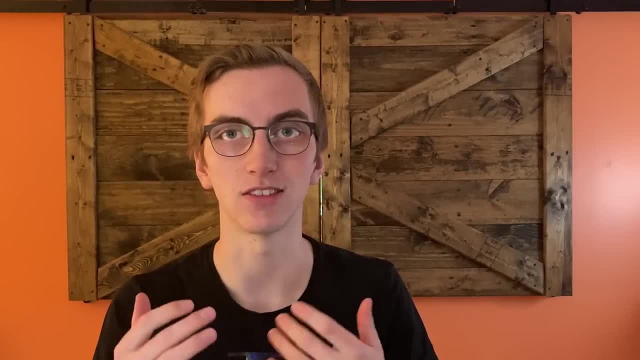 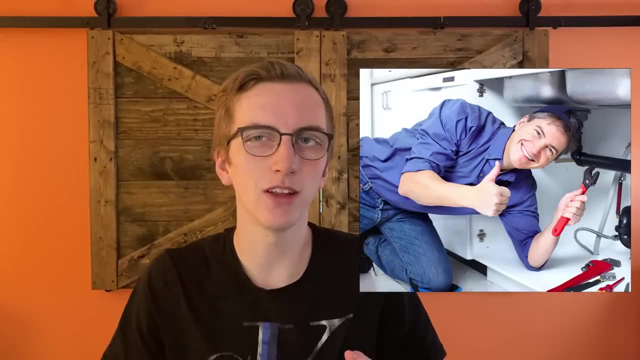 by far your best shot at actually getting employed within a decent job after you graduate. But if you're borderline on engineering and you're not super interested, maybe think about doing something like a trade school and then taking a few university courses that interest you. 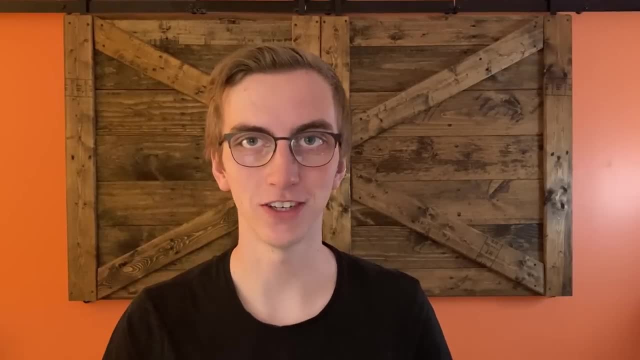 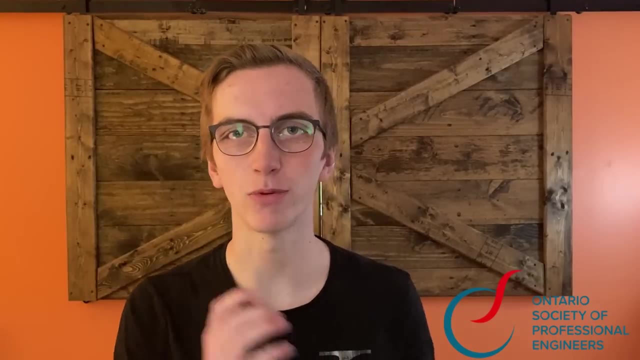 You'll avoid debt and you might actually get a shot at getting a job in your field. So, as these statistics mention, if you're an engineering student, prepare to be disappointed. The Ontario Society of Professional Engineers did a survey asking fourth-year engineering students where they intended to work after. 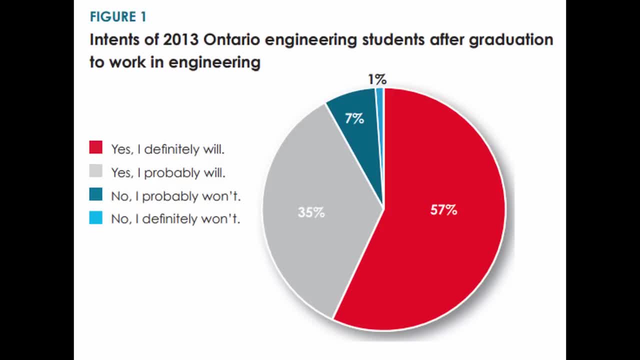 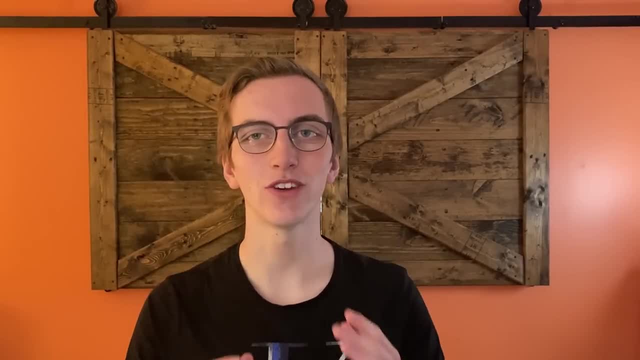 graduation. As you can see, 92% of respondents said that they would probably or definitely be working in engineering, But, as we already know from looking at the statistics, only 25% of these hopeful graduates actually ended up in their field. I'm not gonna lie. this is honestly making 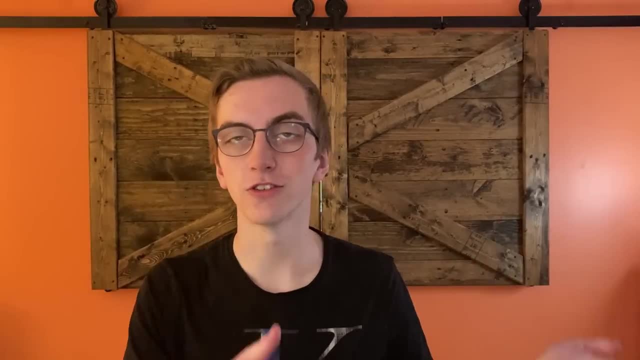 me quite sad, and I don't know who's to blame here. Could it be that universities are not providing engineering students with the skills that employers want to see? Is it the fact that employers are unwilling to work after graduation? Is it the fact that employers are unwilling to work after graduation? 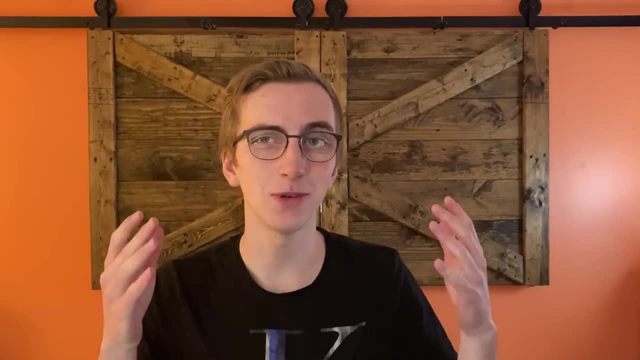 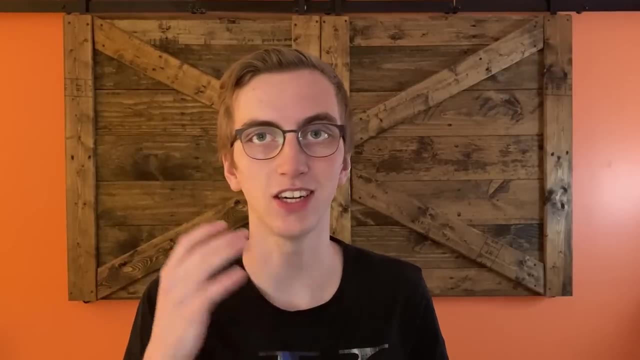 Is it the fact that employers are unwilling to spend money and time to train new graduates? Is the economy simply not producing enough engineering jobs? Or are we just simply printing too many degrees and the rate of job creation can't keep up with it? I think that it's a mix of all of these factors, but I'm inclined to think that the biggest 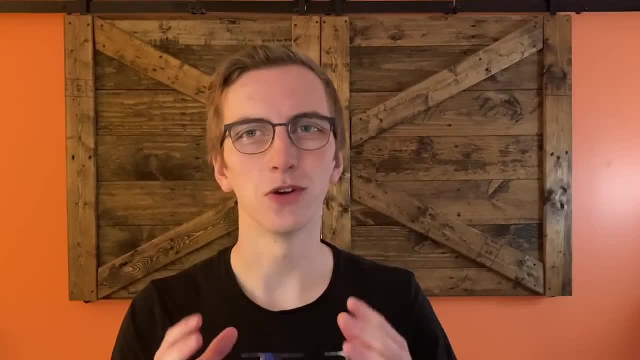 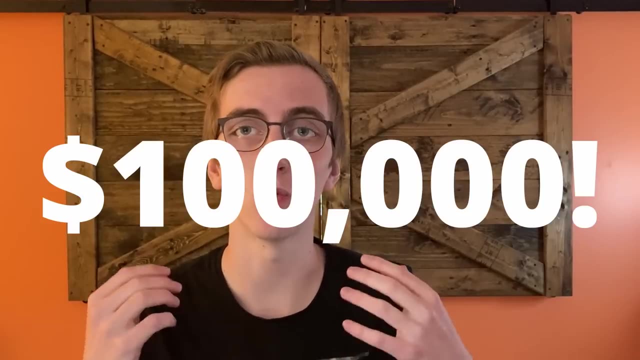 proponent is that there are too many engineering degrees And when you think about this from a financial standpoint, it doesn't really make much sense, because an engineering degree, even in Canada, costs you about $100,000.. So when you think of this from a national or 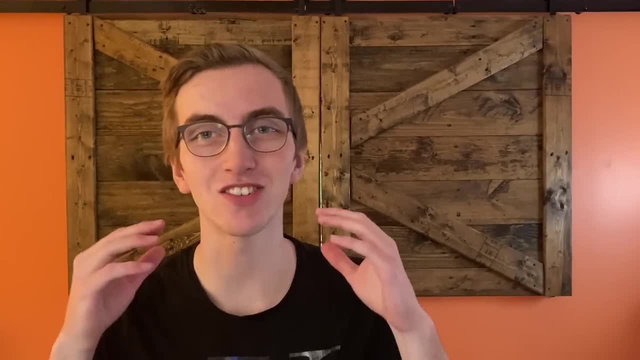 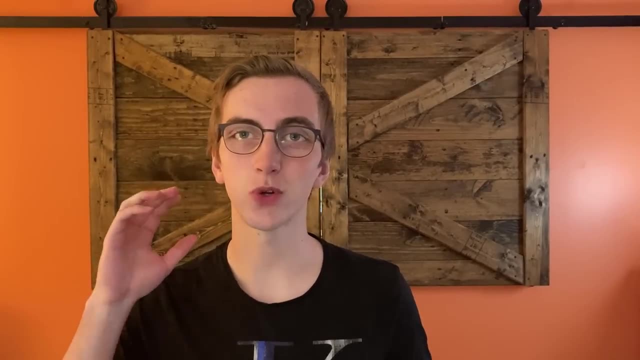 even a provincial perspective. why on earth are we investing so much in the most expensive degrees that we can, when the demand simply isn't there? Engineering degrees are notoriously the most expensive degrees and we're pumping so many students through these programs. for what? 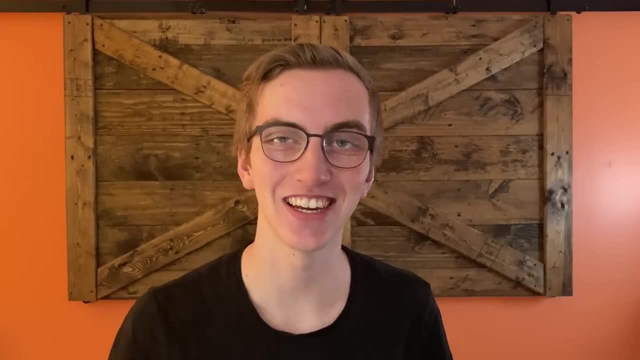 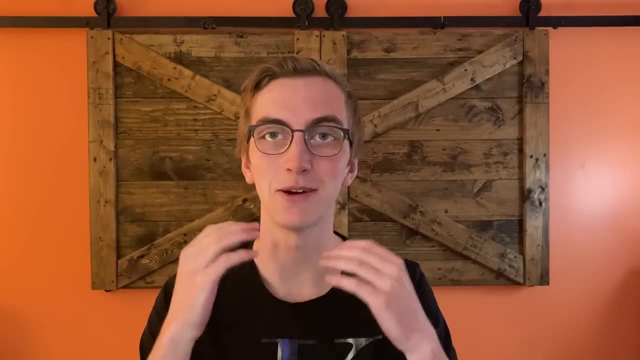 If you were to tell me there was a 25% chance I would actually end up working in engineering, I don't know, maybe I would have rethought doing this engineering degree, Or at the very least I would have spent some more time really thinking about what it was I wanted to do. 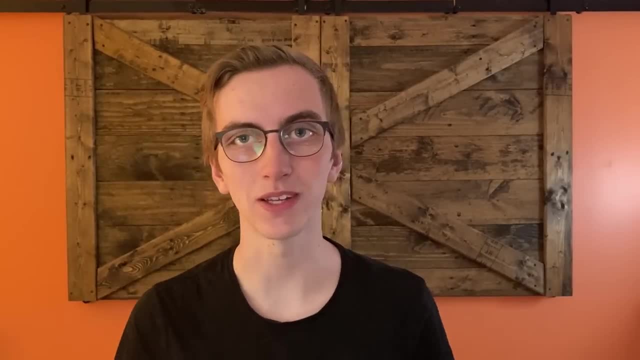 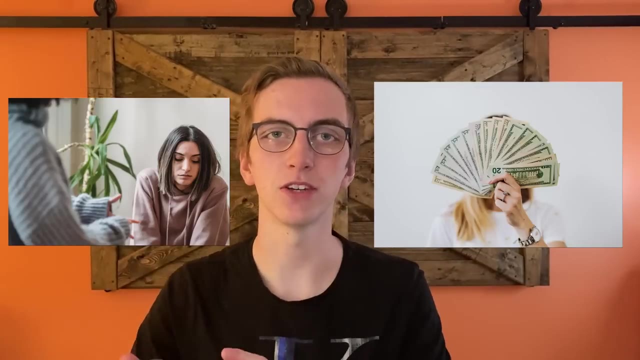 Another common topic that I saw come up, and something I personally believe, is that a lot of people do an engineering degree for the wrong reasons. They might see the nice salary, they might be pushed by their families, or maybe they just want to have the degree for the prestige. 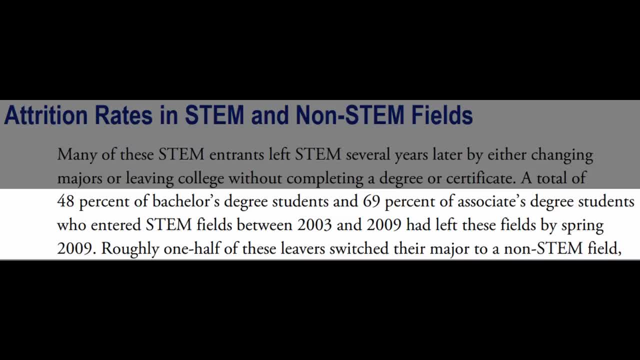 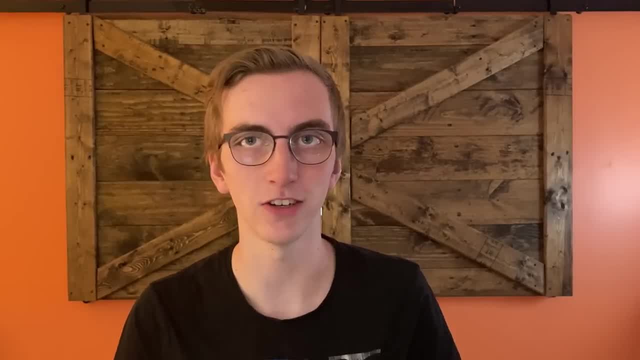 Whatever it is, a lot of students will end up dropping a degree if they're in it for the wrong reasons and, on top of that, those that do stick it out only have a 25% chance of getting a job in their field. And, to make things worse, you have a 25% chance of making your $100,000 investment. 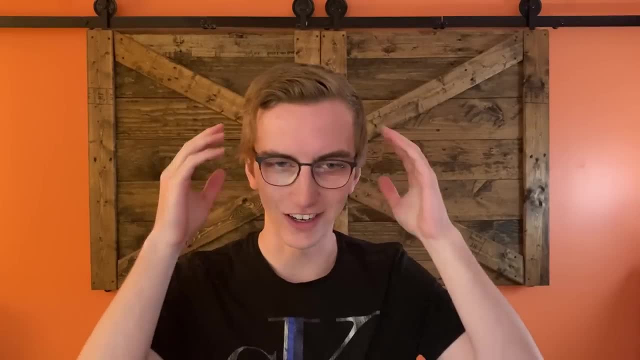 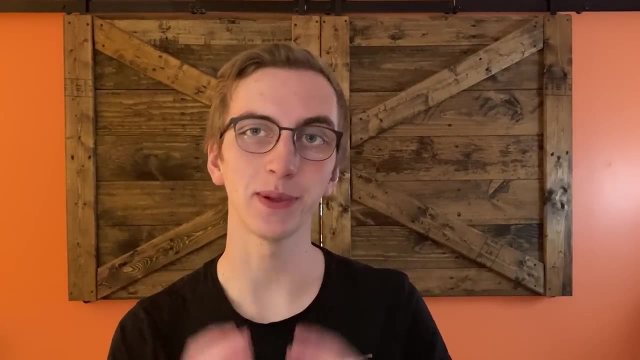 completely worthless by being underemployed. This stuff is honestly insane and it's making me go kind of crazy just talking about it. Alright, look, when I first started my degree, I had the genuine belief that I would be able to work in engineering. no problem, I went to. 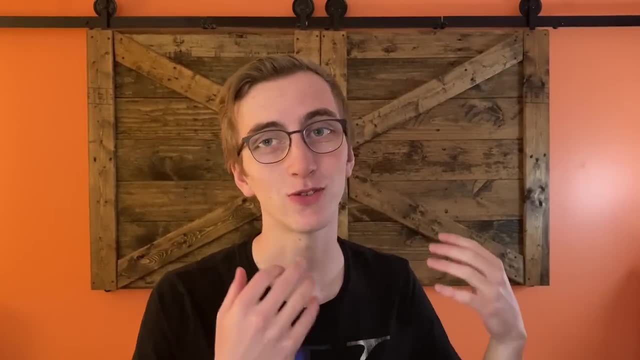 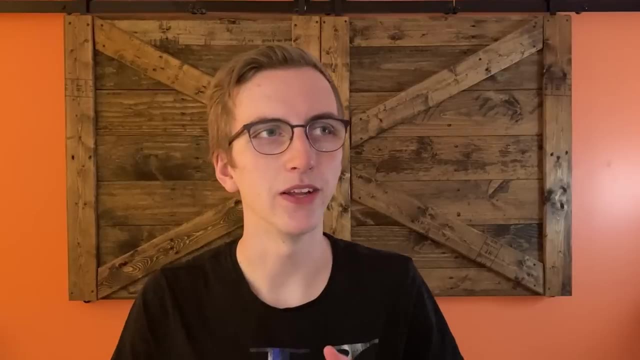 university with the goal of becoming an engineer. However, I'm also super interested in other things like finance, creative arts, music and all of these things I can only call my hobbies right now, But the more and more that I research, the more I start to question why I would put myself through. 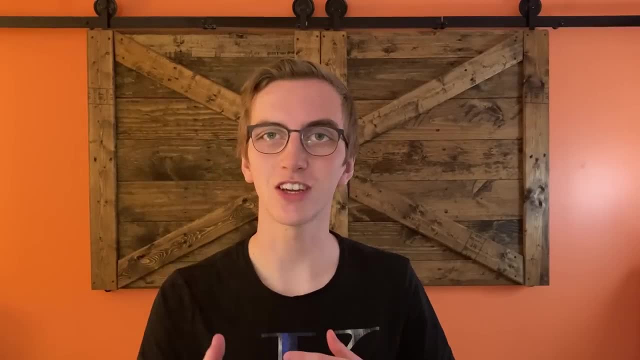 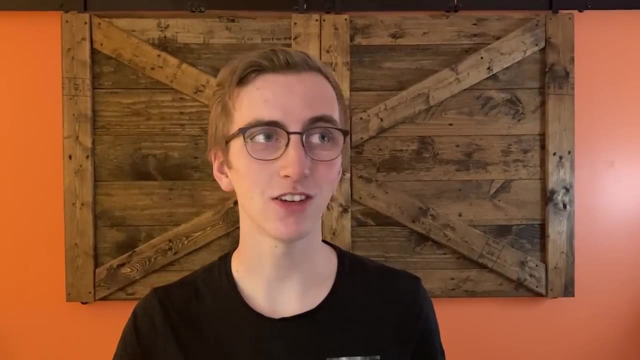 such an uncertain future. I guess in some ways you can look at me and call me part of the problem, because I'm probably going to be one of those engineers who don't end up working in engineering. I battle with myself constantly about whether I should be in engineering, and I can't be the only. 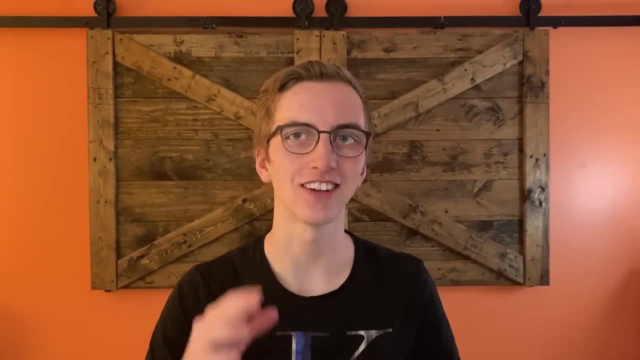 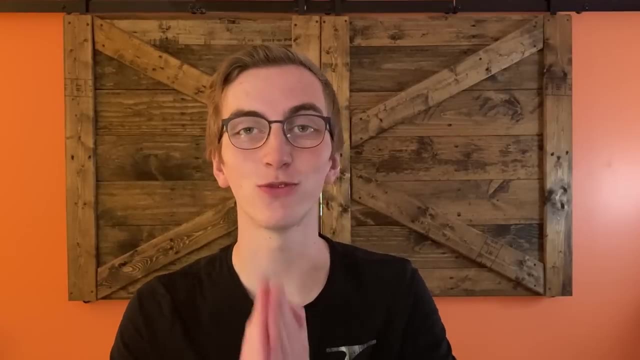 one. I'm sorry that this video turned into a mid-degree crisis. I'll try and save it for a later one. So then this brings me to my next point. Why on earth are we pushing people into these degrees if we know that none of them are going to end up working in engineering? To try and answer, my own question. I'm going to start with the following question: Why on earth are we pushing people into these degrees if we know that none of them are going to end up working in engineering? Why on earth are we pushing people into these degrees if we know that none of them are going to 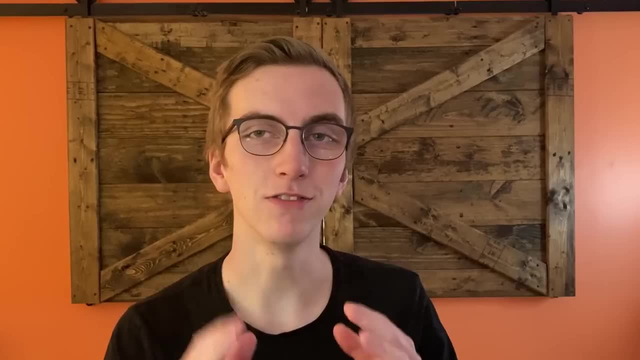 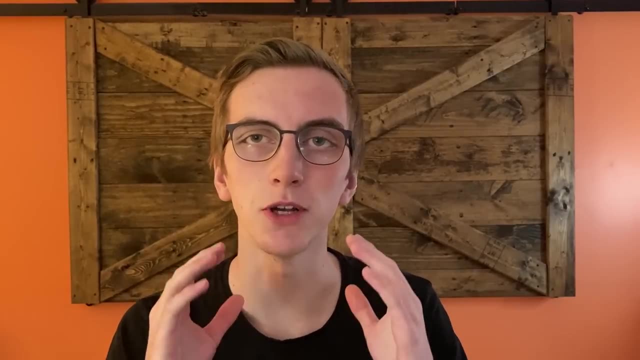 end up working in engineering. Engineering is a great degree for any job. Even though engineers do have a 20-30% underemployment rate, this is still the lowest underemployment rate of almost any bachelor's degree. Alright, so I was listening to this and I got really confused, because why is 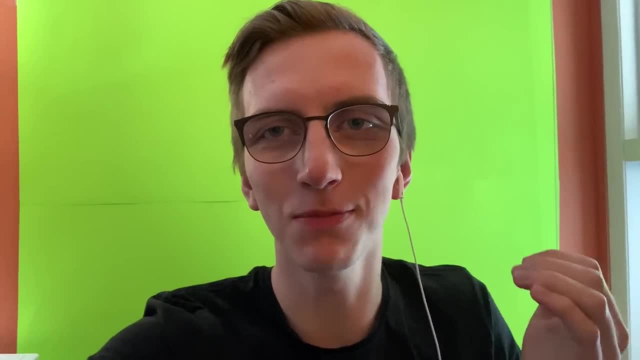 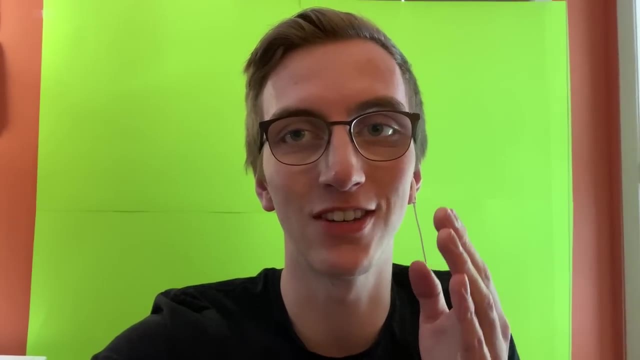 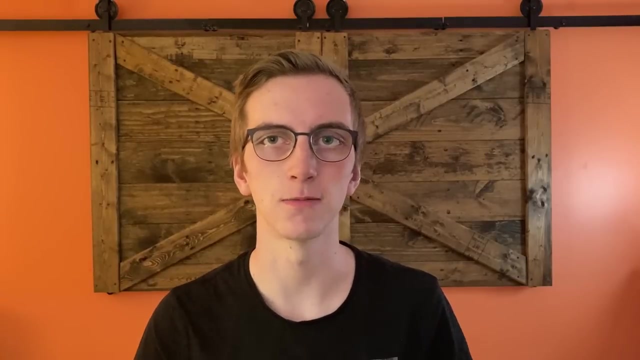 underemployment, the bar, Shouldn't it be something? I-. This shows that there is a huge imbalance between what we're pushing students to go and get versus what jobs are actually out there. This means that overall engineering is still one of the most highly valued degrees, So, ironically, 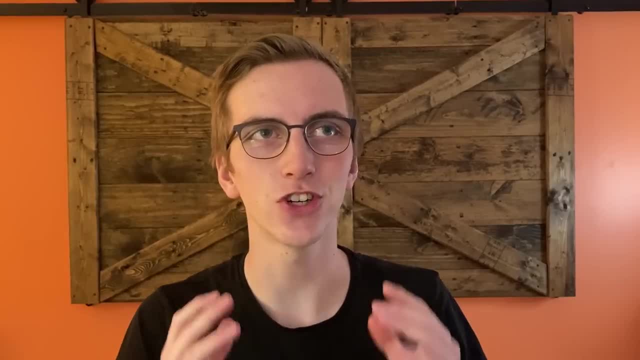 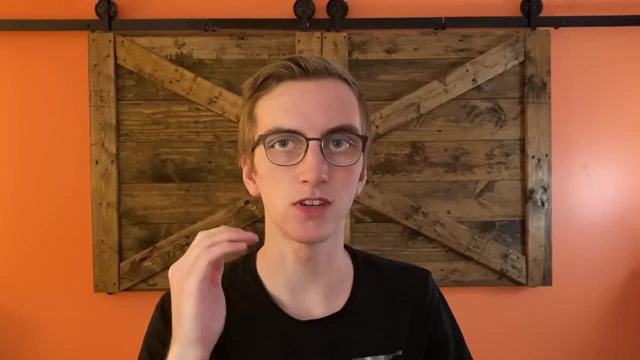 even though there are so many engineering specializations, engineering now has kind of become the general smart person degree. If you're good at math and physics, the next obvious step is to go and get an engineering degree. So I still think that engineering degrees have a lot of. 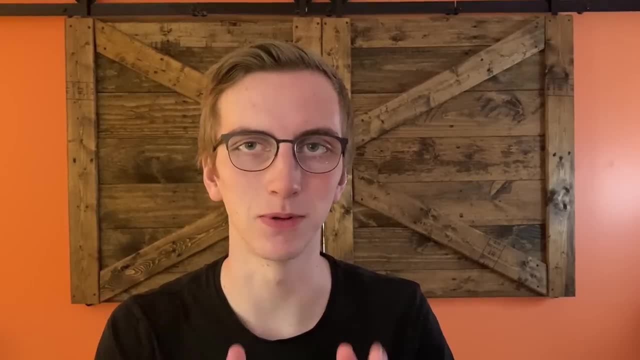 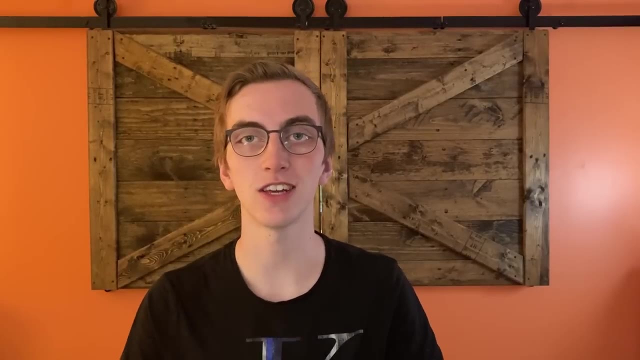 merit, but I don't think that's the only thing we should be telling smart people to go and do. This really is a national crisis across North America and I am going to recommend you stay away from university if you're going for the wrong reasons. I really think that the mindset behind 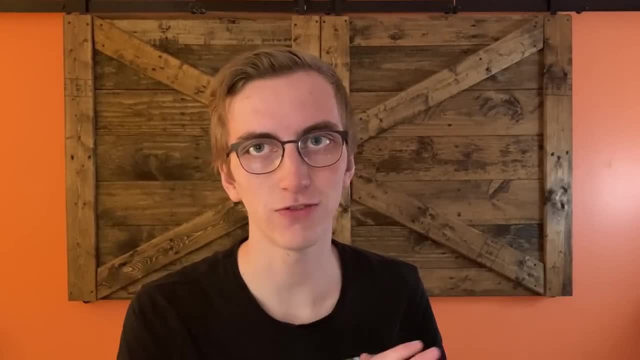 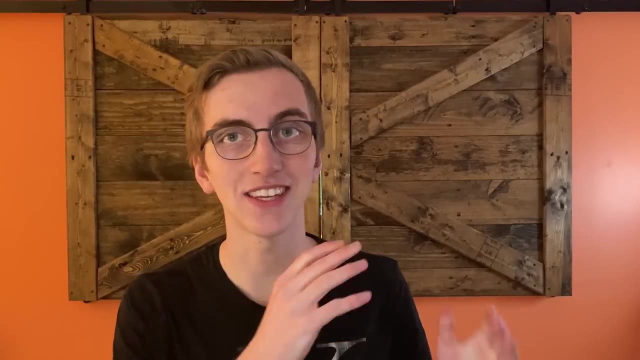 trade schools and more untraditional careers needs to start shifting. These are going to be the careers of the future that provide good jobs, and they already provide really good salaries, And you get the added side benefit of not having to sit in front of a computer 24 hours a day. This video is